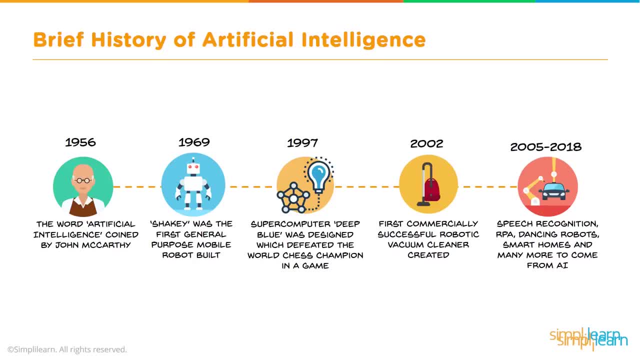 We have speech recognition, RPA, dancing robots, smart homes and many more to come. What I want you to notice about this brief history of artificial intelligence is the compression of time. In 1956 it was just an idea And more than 10 years later we have our Shakey, the first one who's able to flip light switches, And then we go all the way to 97, where we have Deep Blue, And there's a lot of little steps between 69 and 97. But it's actually able to take on a human in chess and beat them regularly. Now they do that in a lot of ways. 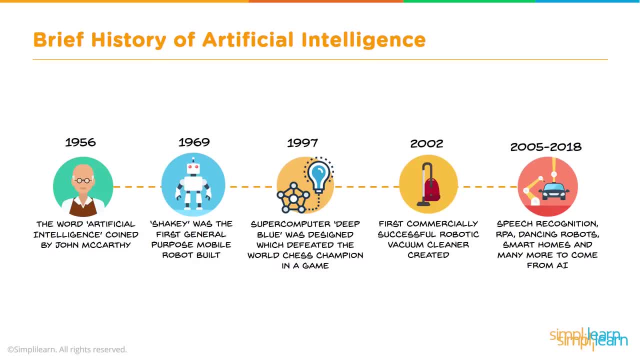 They did have a lot of ties, so don't think that it won every game. And then we go: only four years later, we have our first commercially successful robotic vacuum cleaner And as we go from 2005 to 2018, we go from simple speech recognition to very complicated, able to really register with your Google Voice and your Siri. We have our RPA, we have dancing robots, smart homes and many more things that are just coming out almost monthly in the world of artificial intelligence. 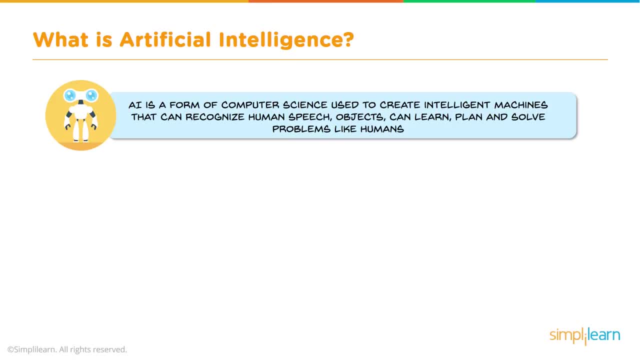 So what is artificial intelligence? AI is a form of computer science used to create intelligent machines that can recognize human speech, Objects, can learn, plan and solve problems like humans, And I'd like you to focus just on that last one. Can solve problems like humans, As we saw earlier. we compare the computer that can beat the chess champion. It's able to the one before that, able to turn on and off lights in the house. So right now, our concept of artificial intelligence is based on artificial intelligence. 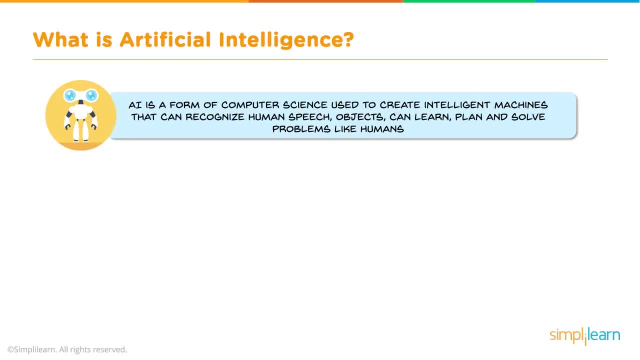 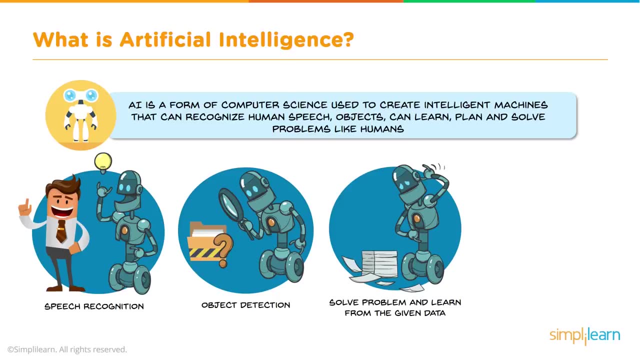 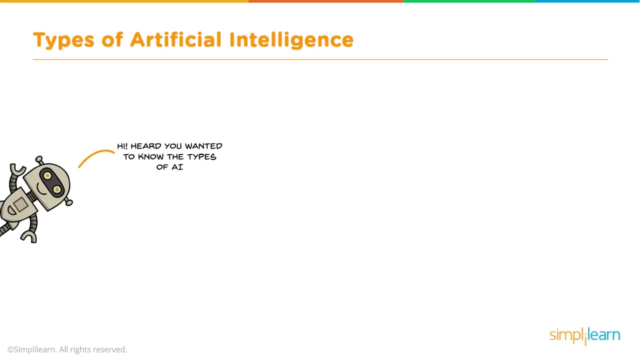 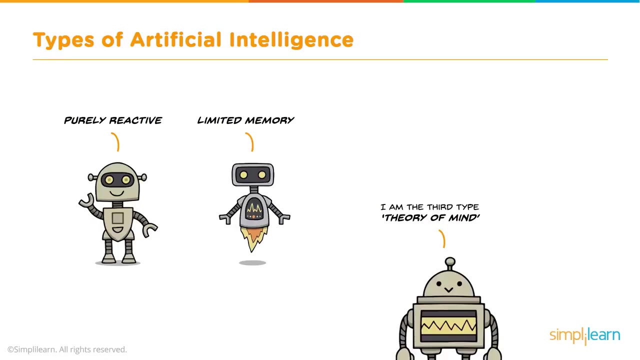 Communication is a very common policy in computer science and teams. Whether in first type is purely reactive, The second type is limited memory. The third type, theory of mind, which is still in the process of being invented, and definitely the question of self-awareness being the fourth, which is still not invented yet. or is it Let's? 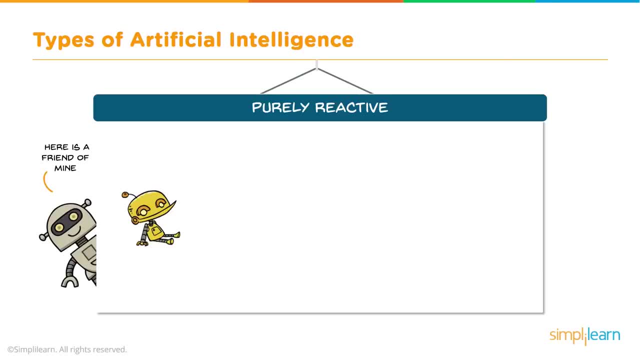 look at these a little closer. Here we have our purely reactive. He does not have any past memory or data to work with. He takes actions, reacts based on what he sees- Okay, it's not that tough- Observes every move. You can see we have a nice game of chess going. 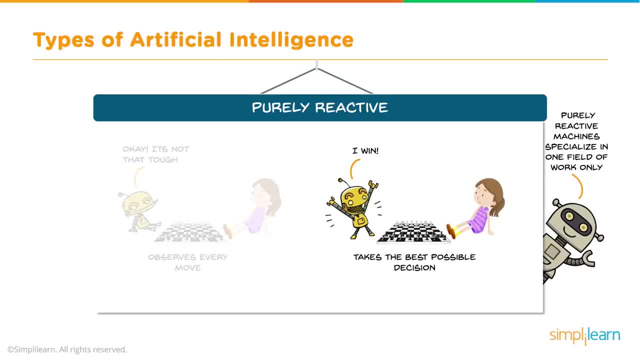 on here And wins, Takes the best possible decision. Purely reactive machines specialize in one field of work only. In this case we see a chess game where they figure out the best moves, calculating all the different moves- Maybe it's calculating the next one. 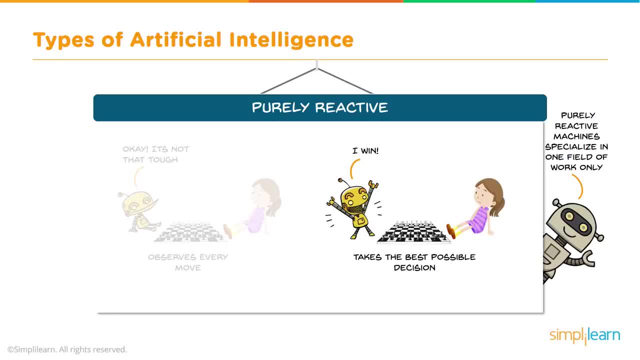 in a row in a linear regression model, so you can figure out the best marketing. But they're very reactionary. They don't have a lot of data, They just have what's in front of them to look at. Next, let's look at limited memory. 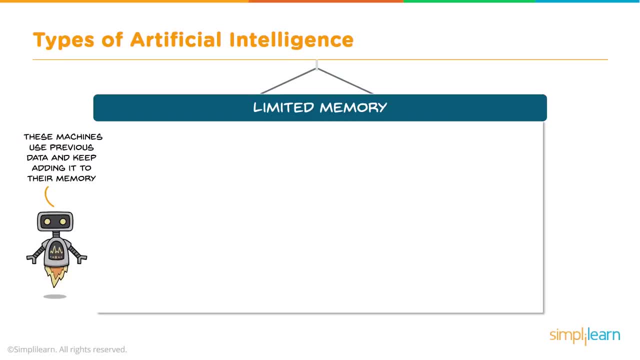 Let's try to understand the limited memory setup. These machines use previous data and keep adding it to their memory. Suggest me a good restaurant. So maybe we're looking to go out for dinner tonight and we're not sure what we want to eat. Hmm, I see you have. 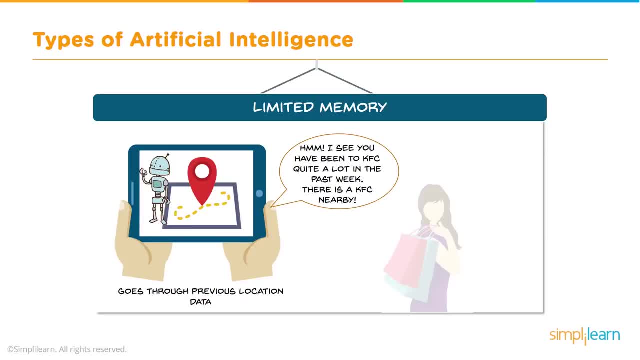 been to KFC quite a lot in the past week. There is a KFC nearby, So it goes through the previous location data and where they ate prior and says, hmm, this is probably a good suggestion for you tonight. Thanks, It has enough memory or experience to make. 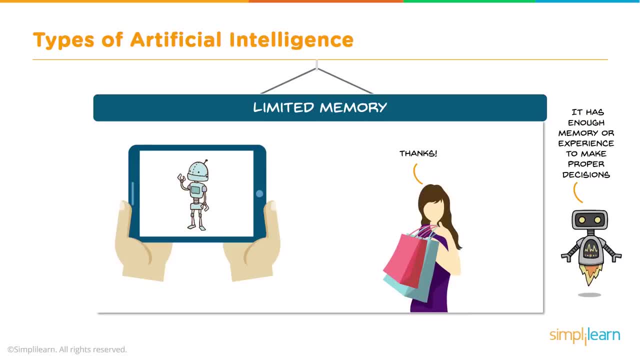 proper decisions. But the memory is very difficult. It's hard to understand. And it's hard to understand, It's very limited. This isn't trying to guess what a new location would be or anything like that. It just takes what it has in front of it and goes: okay, this. 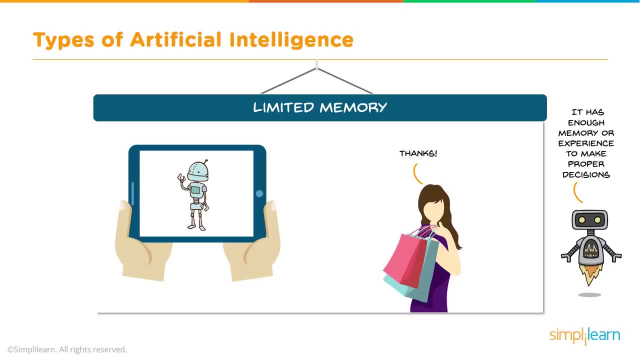 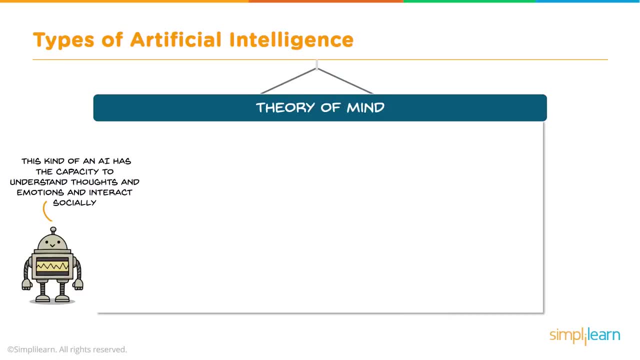 is where you've been. This is what you liked. You gave it two thumbs up, one thumb down, whatever, And then it goes from these suggestions. this is where I think you should go. Theory of mind: This kind of AI has the capacity to understand thoughts and emotions and interact. 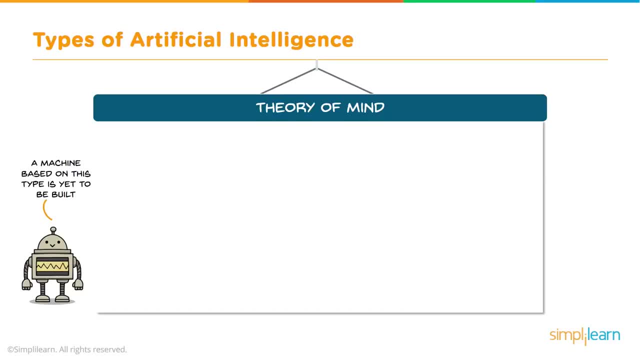 socially. A machine based on this type is yet to be built. That human looks lonely. Hey human, you want to be my friend? Huh, Okay, Theory of mind is a thing of the future. Certainly, we see a lot of the industry. 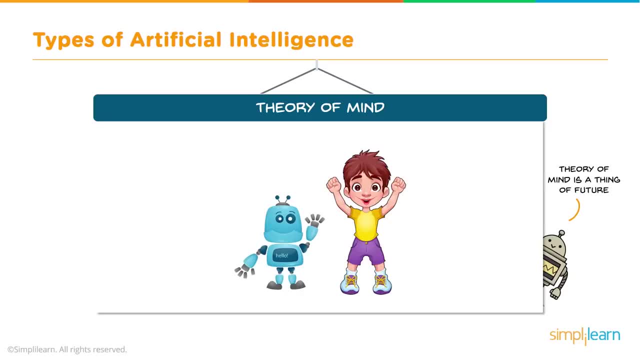 poking a little bit at this, as it tries to guess how you feel about things, But most of that is still based on previous data, You know? yes, no, two thumbs up, one thumb down. Theory of mind would take it one step further in understanding the emotions behind it, And 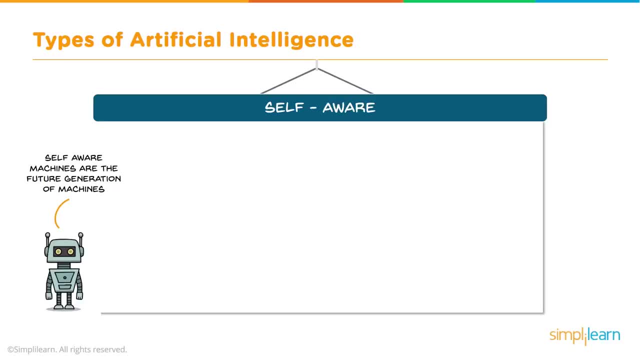 finally, as we get deep into the sci-fi, futuristic, we have self-aware. Self-aware machines are future generation of machines. They will be super intelligent, sentient and intelligent, Okay, Like the Terminator, the good guy in the thing, or Ultron, or Vision from Avengers, For right. 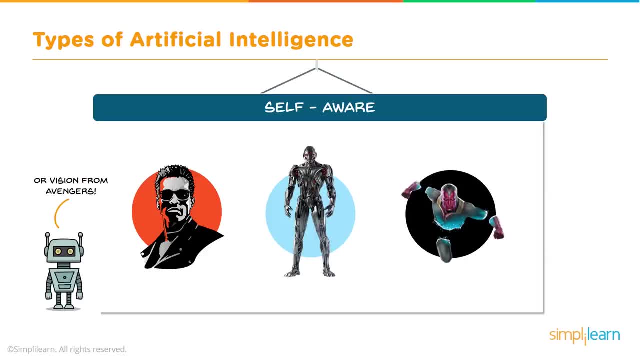 now these are mostly movie characters or cartoon characters, but we certainly are getting closer to seeing them in the real world. Hopefully they'll be of the type of the good guys and not the bad guys we see also in the artificial intelligence, sci-fi movies. 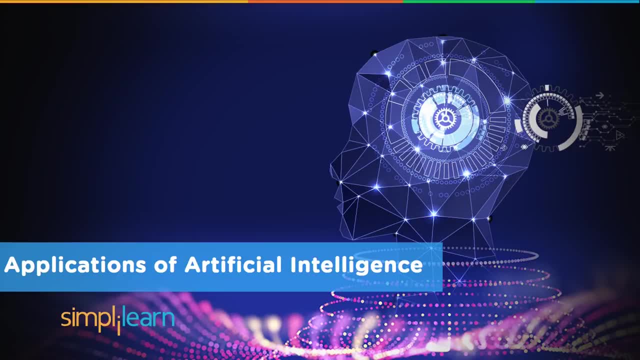 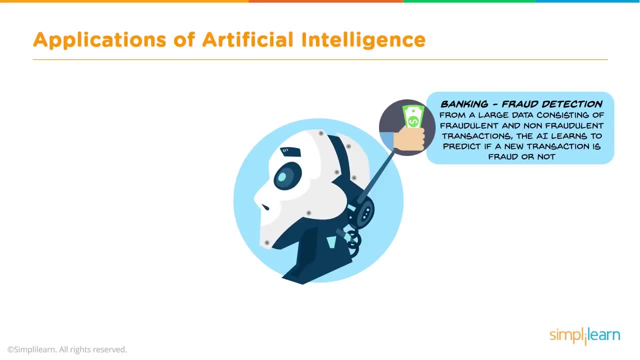 Applications of artificial intelligence. Let's take a look at some of today's commercial and business uses for the AI. We have banking fraud detection. From a large data consisting of fraudulent and non-fraudulent transactions, the AI learns to predict if a new transaction is fraud or not. 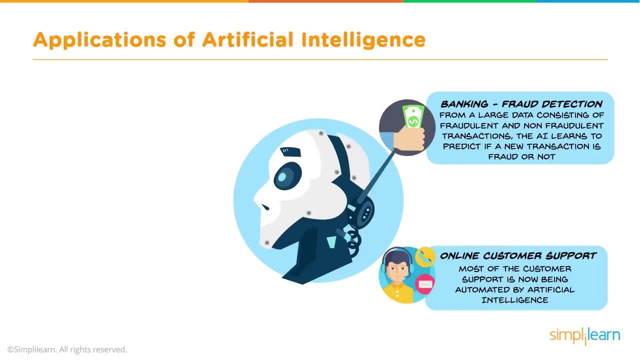 Online customer support. Most of the customer support is now being automated by artificial intelligence: Cyber security, Using machine learning algorithms and a lot of sample data. AI can be used to detect anomalies, adapt and respond to threats. Virtual assistants, Siri, Cortana, Alexa and Google now use voice recognition to follow. 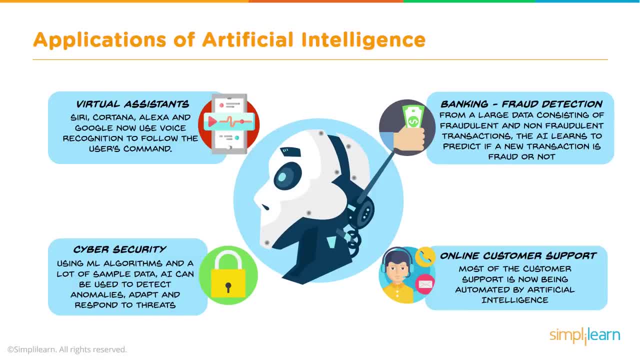 the user's commands. These are all wonderful examples of current AIs that are in the commercial and business world, and these ones in particular have matured over the last half a decade. For instance, very few large banks in today's world would not use banking for fraud detection. 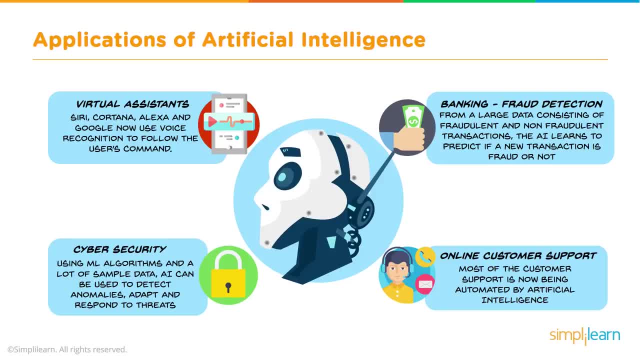 or for deciding whether it's a good person to give a loan to or not, based on their credit scores and where they're from and their income. Same thing with cybersecurity, detecting anomalies or online customer support. Could you imagine in, say, HP, who has over 70,000 help pages across 17 different languages? now they have to figure. 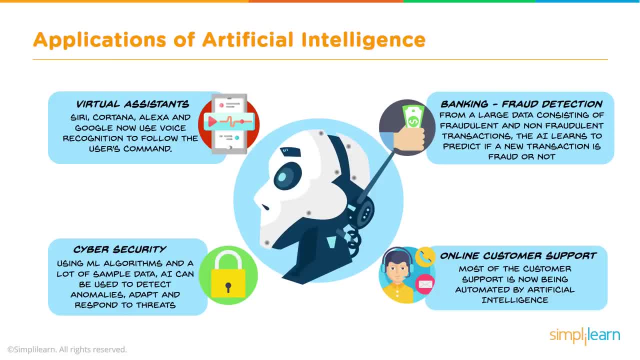 out how to do online customer support to cover new problems that come up and track them so they can build new pages. If they had one person doing that, that would take them a year just to do what they need to have posted yesterday. And, of course, our virtual assistants. I don't know about you. 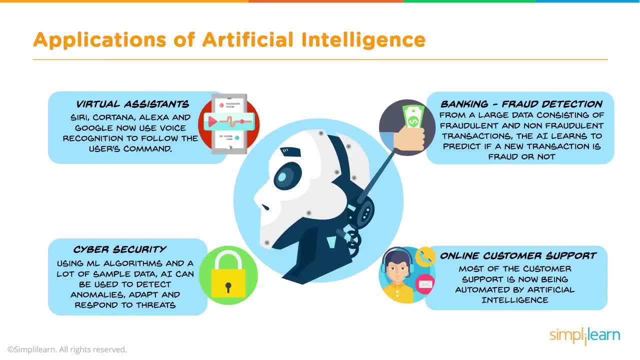 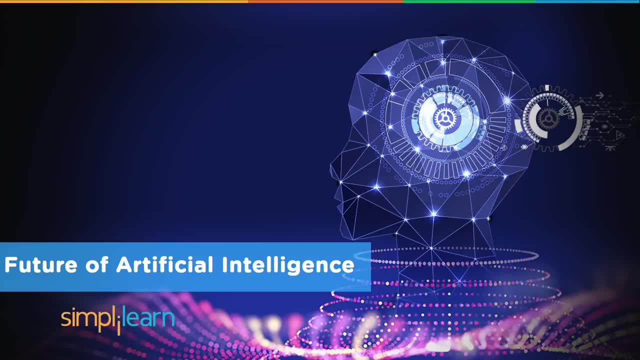 but I love mine, kind of like having a private secretary without having a private secretary. Future of artificial intelligence: If we see where it's at now commercially and business-wise, then where is it going. Of course, the imagination is a limit on this one, but you can already see.